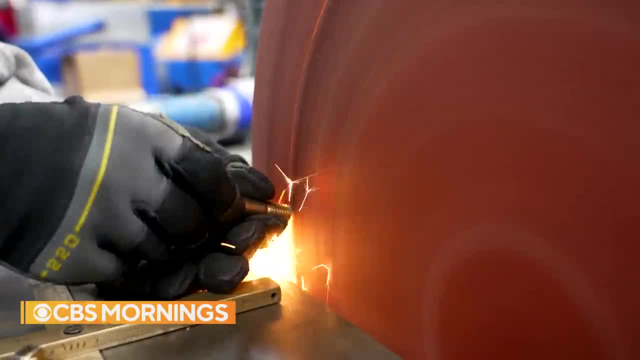 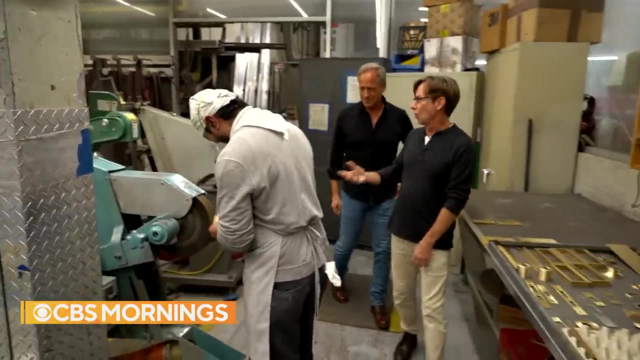 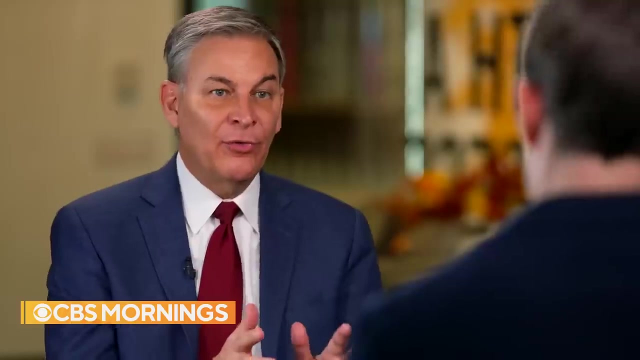 Do nothing. Rowe and I met at Empire Metal, a fabrication and finishing shop In Queens, New York, And where, much like manufacturing shops nationwide, finding skilled workers like these is a growing challenge. We have more jobs than we have people for. 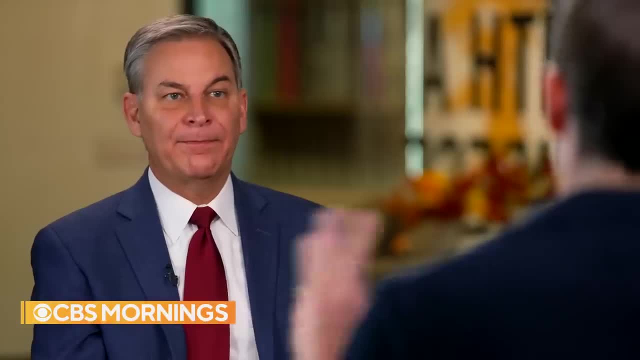 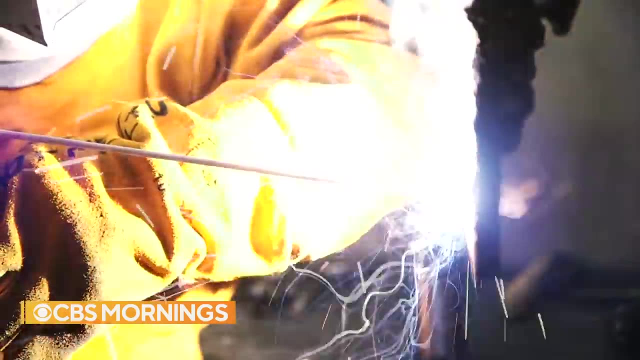 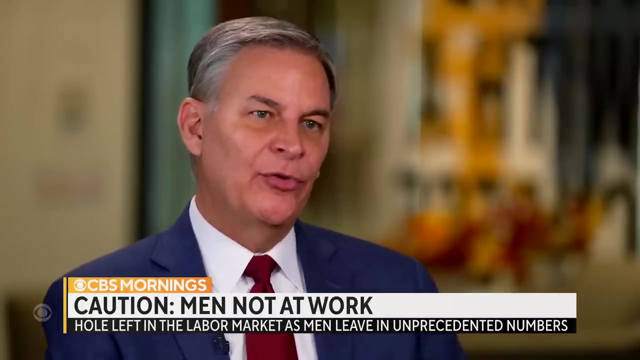 About one and a half jobs for every one worker. Jay Timmons, who leads the National Association of Manufacturers, describes all this as a profound problem for the companies he represents. 99.9% of them will say that their number one challenge right now is being able to fill those open jobs. 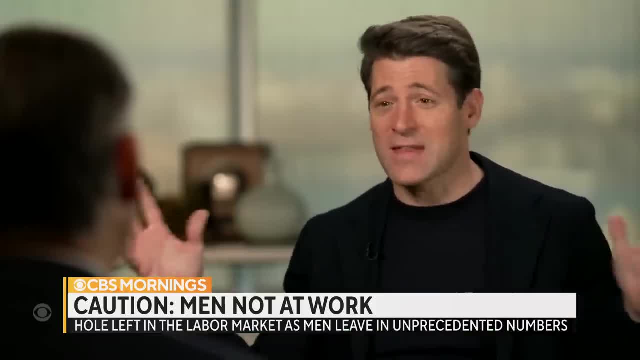 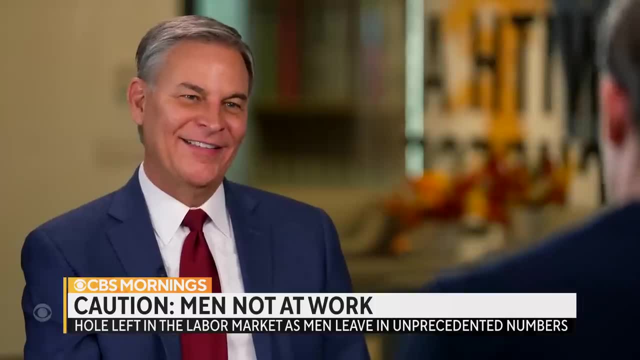 So you are here as a representative of more than 14,000 manufacturers in these United States, And the number one problem for 99 out of 100 of them is filling jobs. Yeah, I never thought I'd be able to say that. 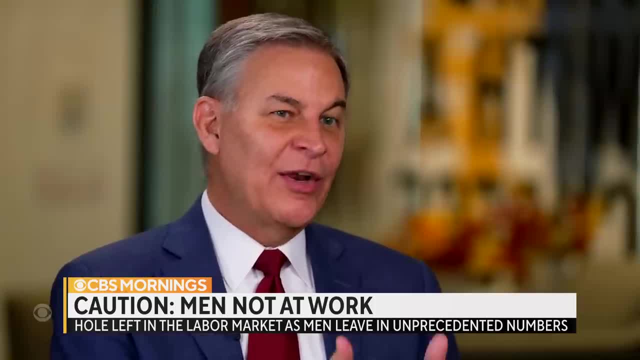 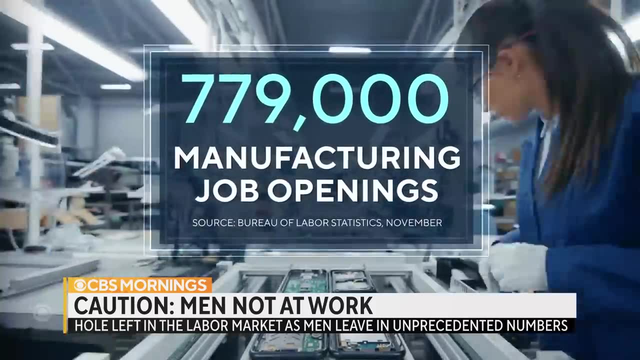 But now it's kind of an all-hands-on-deck. We've got to fill these jobs that are open, And there are nearly 800,000 of those jobs open right now, according to the latest federal count, a number that surged in recent years as companies 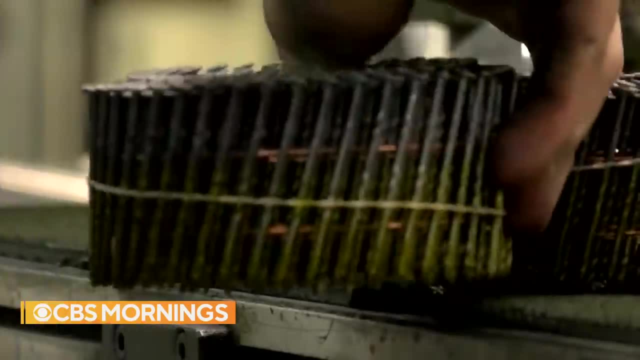 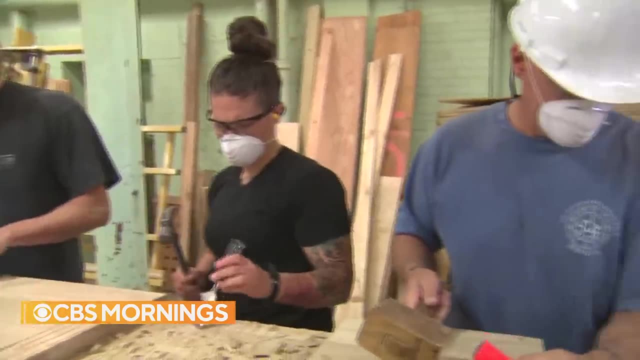 reinvest in American-made products or try to anyway, And with manufacturing workers earning more than $30 an hour on average. Timmons says the problem is not pay but perception. It used to be dirty, dark and dangerous. Today it's very sleek. 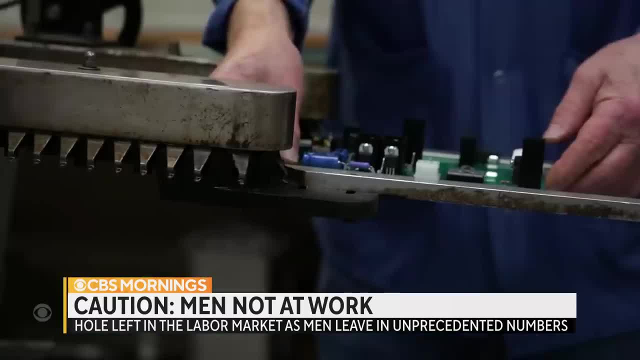 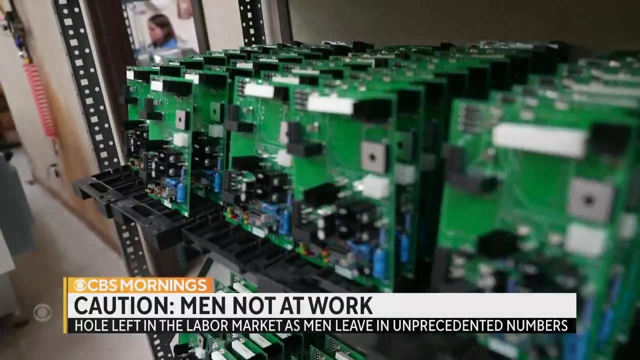 It's very technology-driven, And that's what we saw when we visited Electrosoft, a company outside Philadelphia that makes circuit boards for everything from missiles to submarines. So over there is the quality area. Okay, Okay, Okay, Okay, Okay. 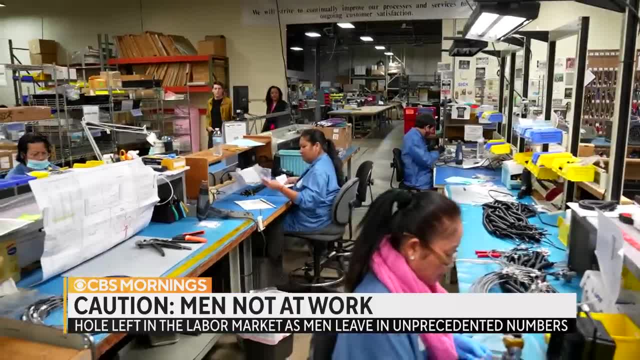 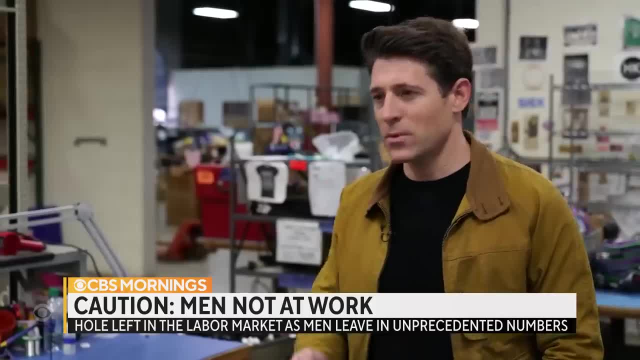 Okay, We do first-piece article testing, final testing. But CEO Carla Trautman says they could be doing more. if only she had the workers to do it. How many people work here right now? Thirty. How many people do you wish worked here right now? 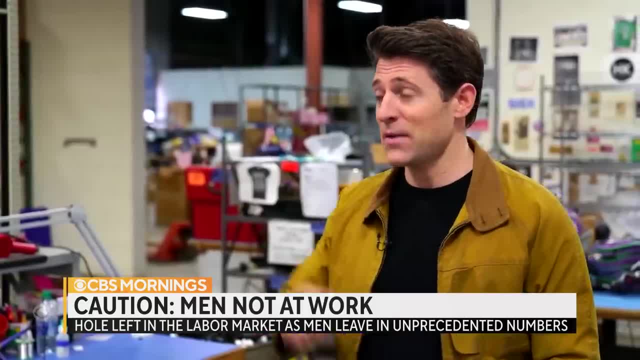 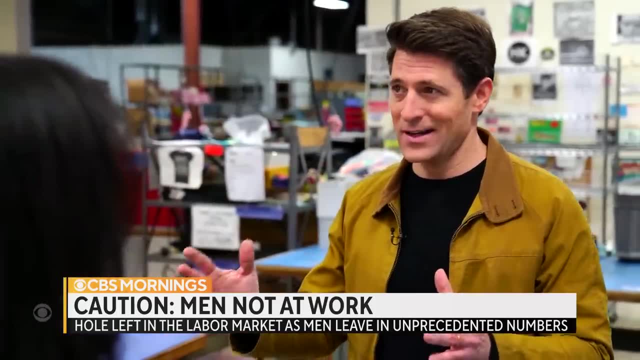 Forty-five. So you have 15 people that you have jobs for, Yes, But you can't find them, Cannot? How much money in lost business is there in not being able to hire the people that you want? Around five million. 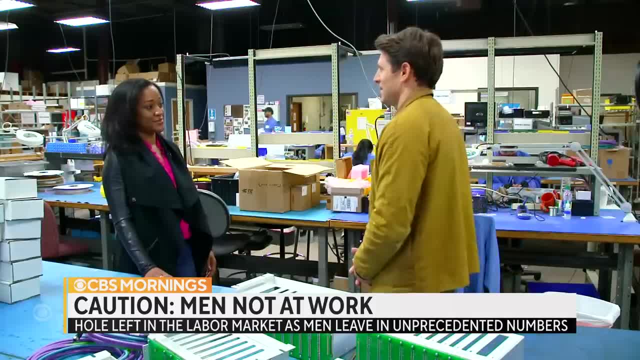 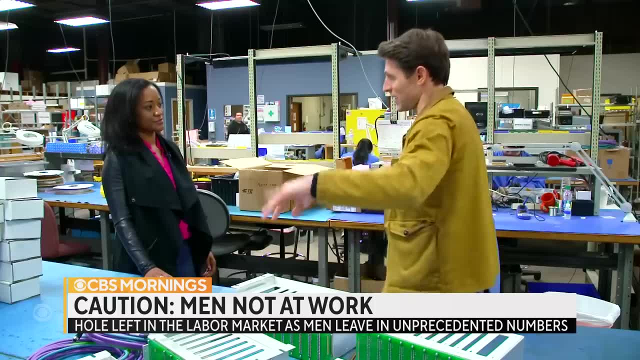 In top-line revenue Five million? Yeah, That would be here and that presumably you'd be paying taxes on. Obviously, yeah, And that would go into people's pockets and would be going out into the broader economy. Yeah, What is your theory about where those 15 people are right now? 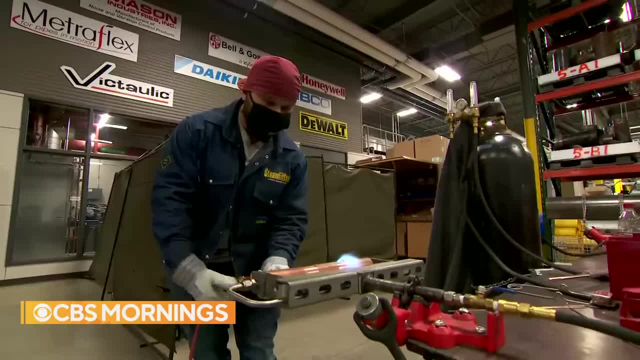 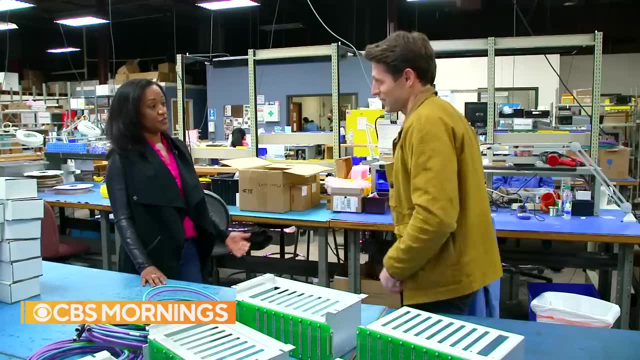 I honestly have no idea where they are. She suspects some people may be sitting out because of a recent change in the way many of us look at work. I think it's fulfillment, I think it's culture. I think people really want to feel as though they are working. 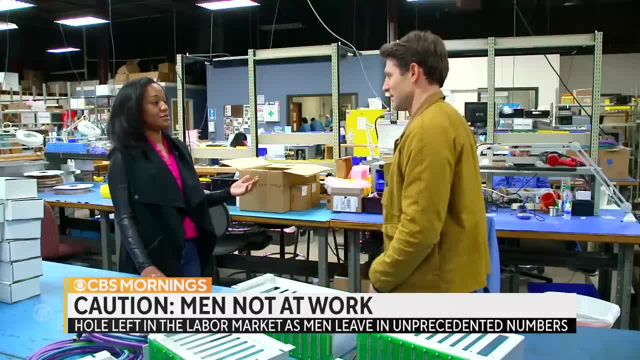 I think it's fulfillment, I think it's culture. I think people really want to feel as though they are working. I think people really want to feel as though they are appreciated. I mean Beyonce's song. she said: release your job. 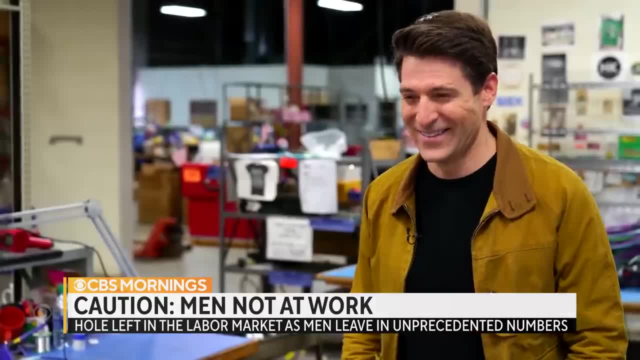 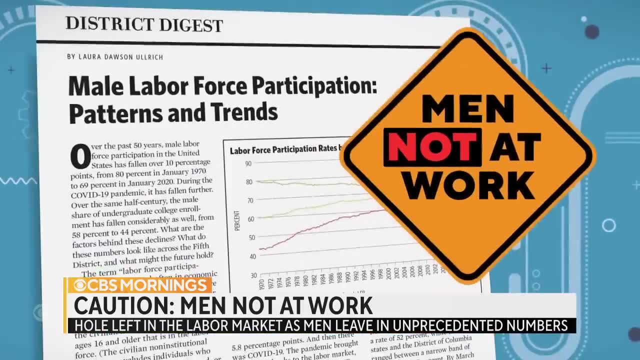 A lot of people release their jobs And they realize. I mean it's an overall feeling of being fed up, Yeah, And being taken for granted. But there's more. According to one economist, some non-working men face a skills mismatch. 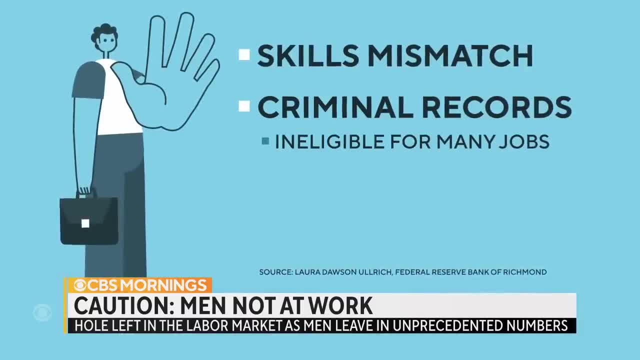 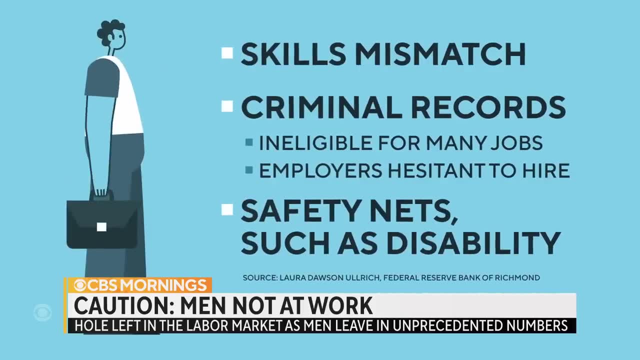 A third have criminal records making them ineligible for many jobs and making employers hesitant to hire them, And many rely on safety nets such as disability. So you may wonder: what are these guys doing instead of work? Well, kind of what you might expect. 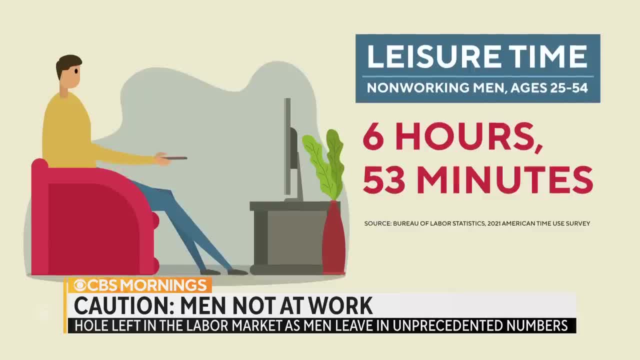 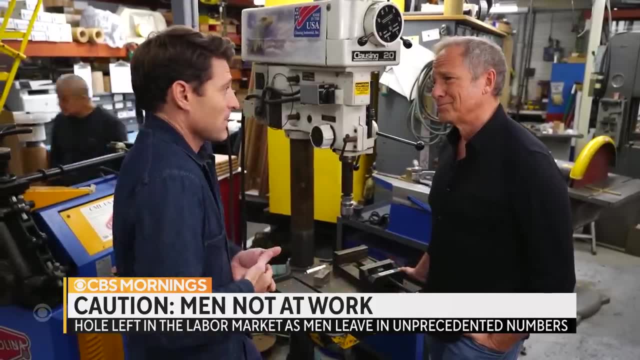 Spending nearly seven hours each weekday on average, relaxing, playing games and watching TV. So how is it from where you're sitting, from your understanding that people can do nothing all day and still have enough money for a bag of chips? 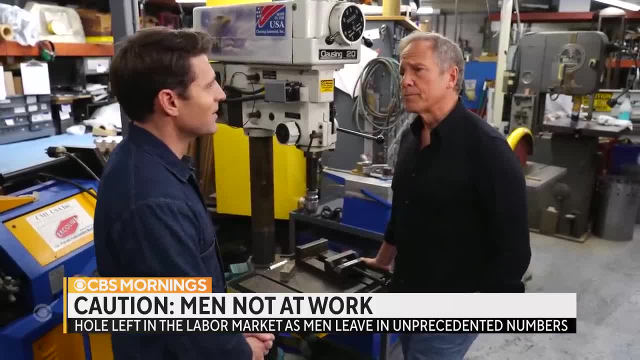 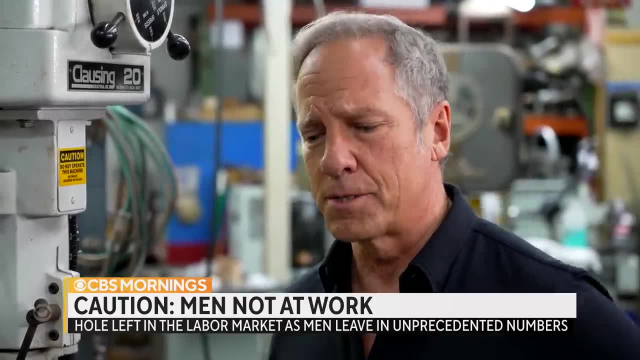 Oh well, it's almost as though some entity is paying them. It's almost as if somebody is not letting them fail. It's as if some giant parent somewhere has An uncle. maybe Could be a rich uncle. yes, Could be a very wealthy uncle. 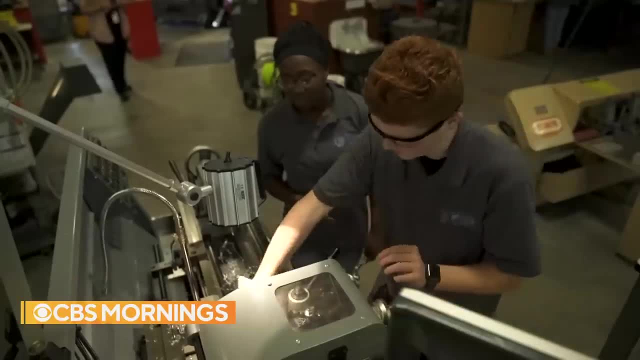 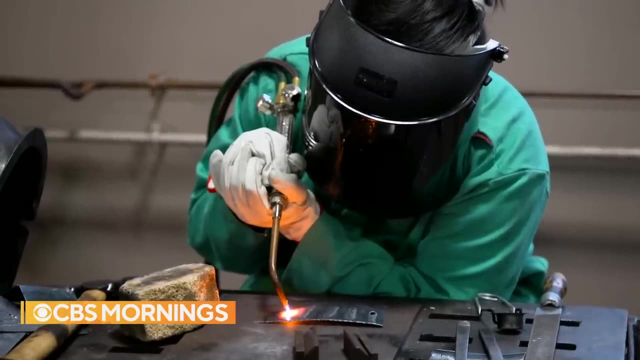 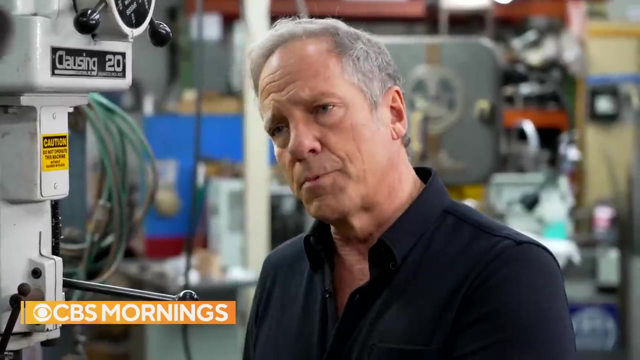 Or it might come down to values, As many public schools have stopped offering shop class. many students have stopped even considering jobs like the ones Roe has spotlighted, Dirty or otherwise. It goes back to the stigmas and stereotypes and myths and misperceptions. 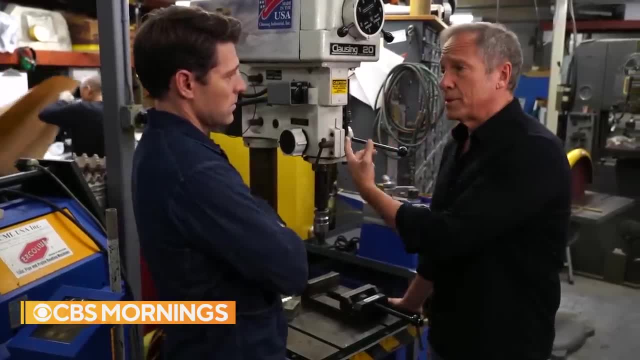 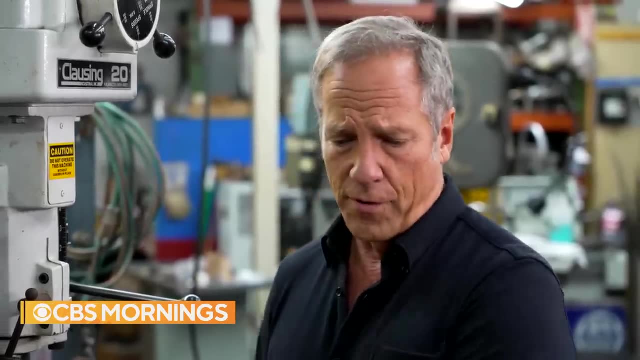 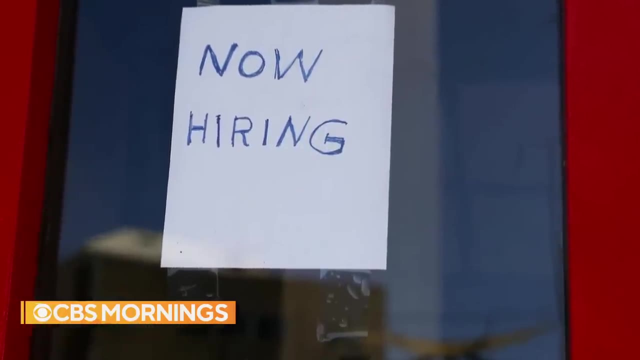 keeping guidance counselors from talking about opportunities like this to the kids in their care. It's those things that are keeping parents from putting all the options on the table. How big of an issue is it to have this many people sitting on the sideline? It's only a matter of our national identity. 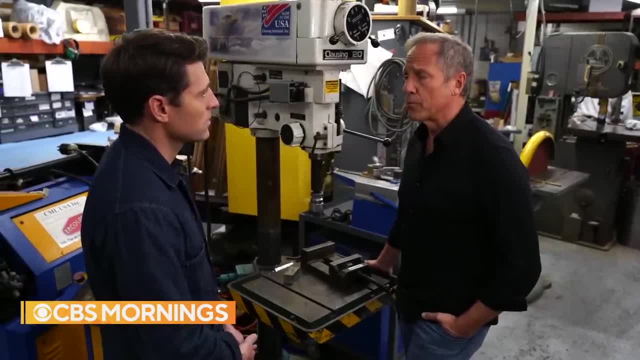 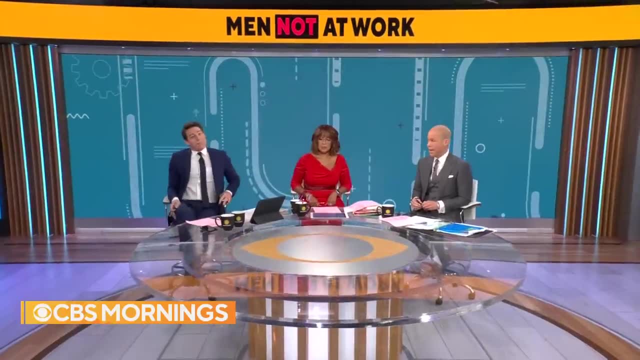 I think it's a giant issue And by the time we realize how big an issue it is, we're going to have a hard time turning the temperature down. It's a fascinating story: Seven million men and they're watching seven additional hours of TV and relaxing. 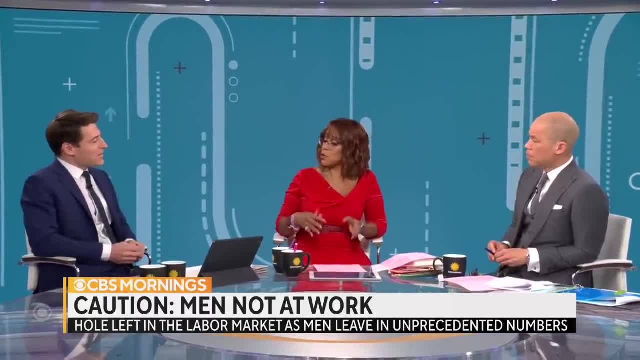 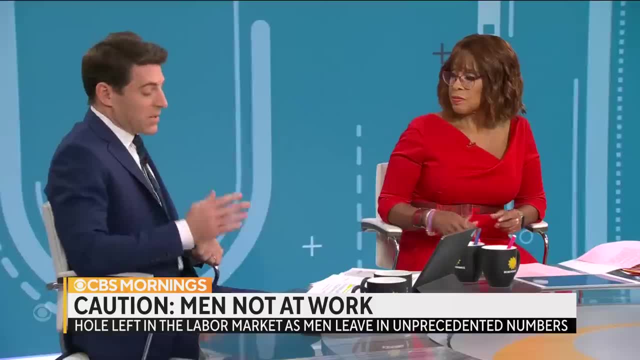 Yeah, that figure got me. Are the women in their lives? are the partners in their lives working? So this is where it gets a little bit political. People on the right will say these guys are just living off government largesse, They're getting disability, they're benefiting from aid and that's got to be reformed. 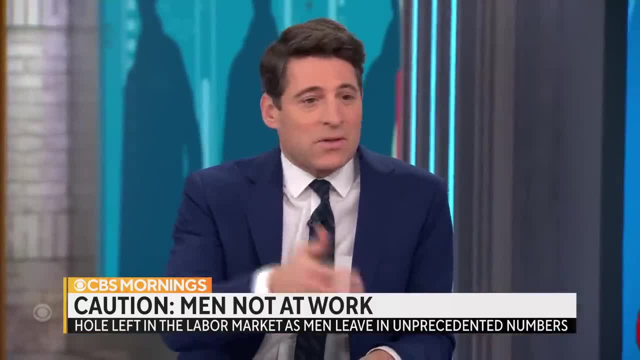 And people on the left say they just need to be trained up And yeah, in the meantime they're living at home or they're depending on partners. You mentioned this skills mismatch And it just made me think. you know, my grandfather was a machinist. 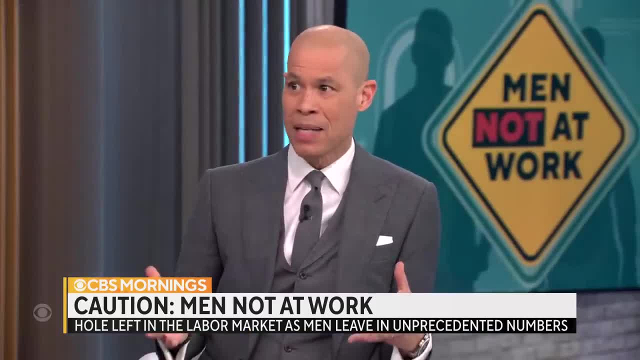 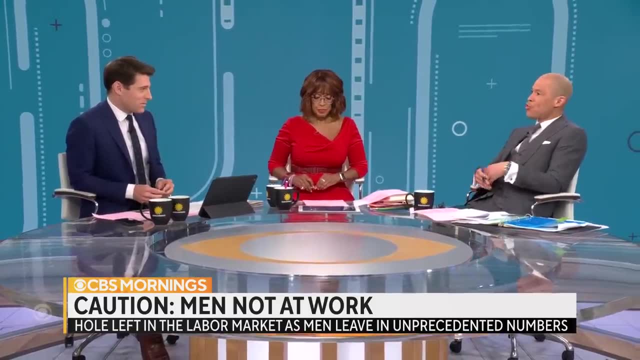 Which Is a highly skilled job- Not anybody. You have to be trained to do that And I don't know a lot of machinists now in 2023.. And I wonder if people are being trained for that. And he mentions Mike. 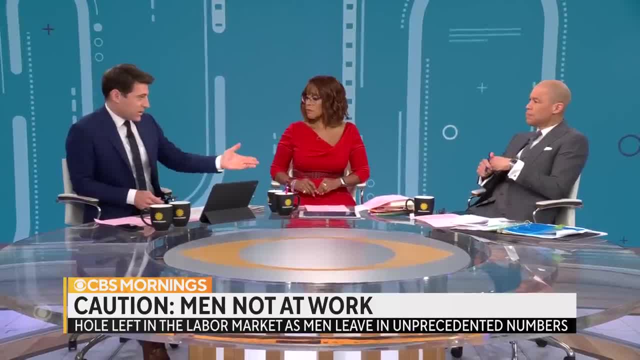 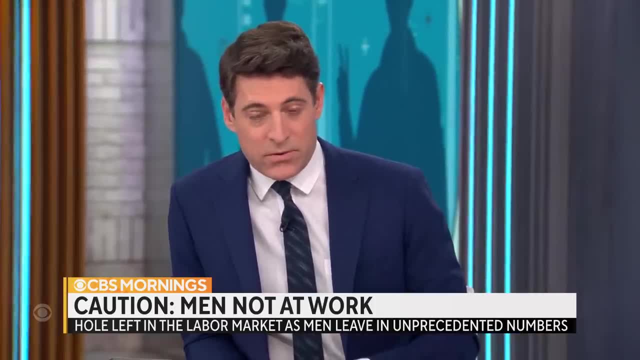 So Mike Rowe has a foundation called Mike Rowe Works where he does give people scholarships for that kind of training. That's part of the issue. But like Carla Trotman, the woman in Philadelphia who runs the circuit board manufacturing facility, she'll train you herself. 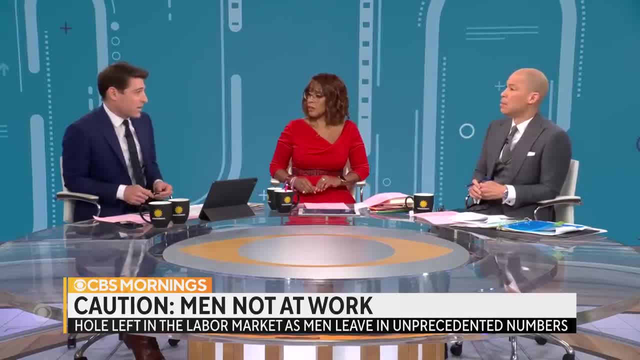 If you're in the Philadelphia area, they're looking for 15 people there. It pays well. It's a nice, clean, quiet place to work, So go there. By the way, some people think, oh, maybe these guys are doing more stay-at-home dadding. 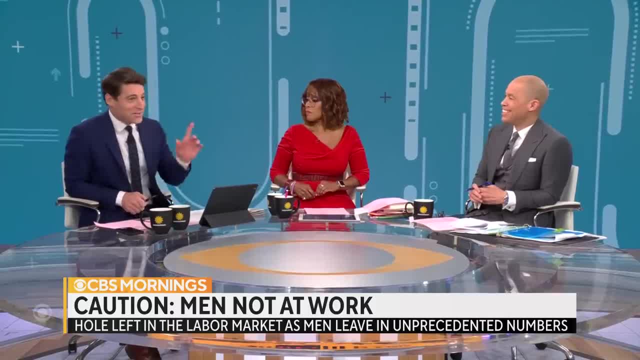 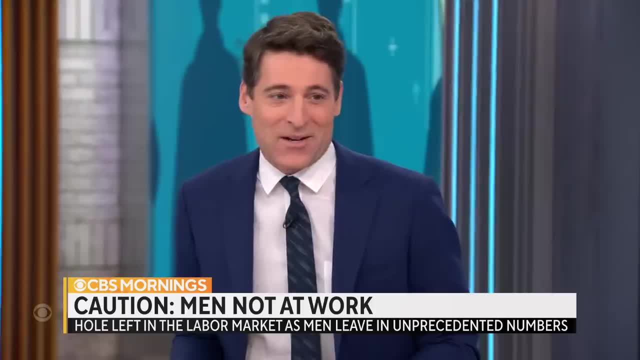 That's an optimistic point of view. They're not. I looked at the numbers. Shauna Thomas, our executive producer, brought this up. In fact, these guys who are not working and not looking for work are spending less time caring for other household members than the guys who are at work. 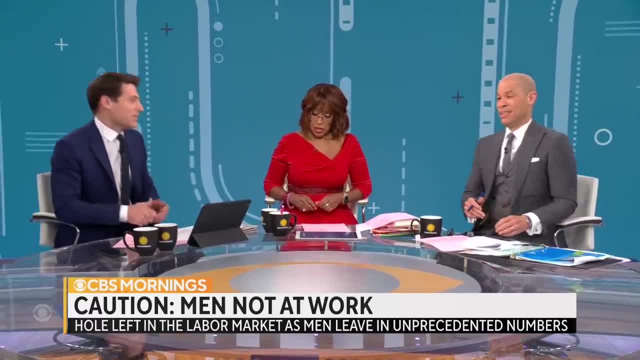 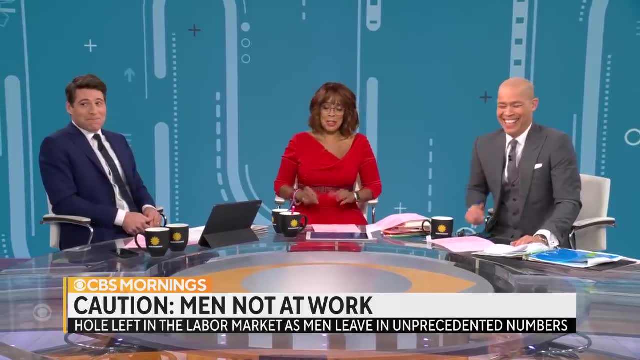 So they're doing less childcare, not even a little bit more, I don't know. But an able-bodied man who can work, and doesn't? it's not attractive. I was just going to say not attractive, And on that note, Okay, I'm just saying for a friend.